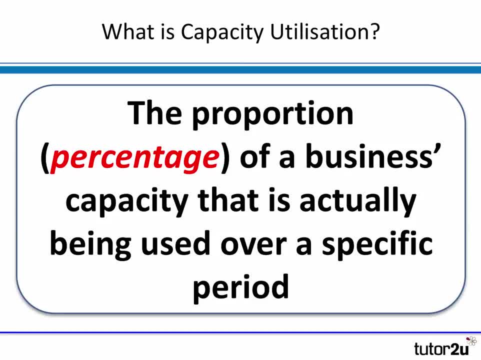 match. So capacity is a measure of output, Capacity utilisation is a percentage, So it's a percentage calculation. And what it does? it compares the actual output that is produced or used compared with the potential. So capacity utilisation, you clearly need to know both the actual output, but also. 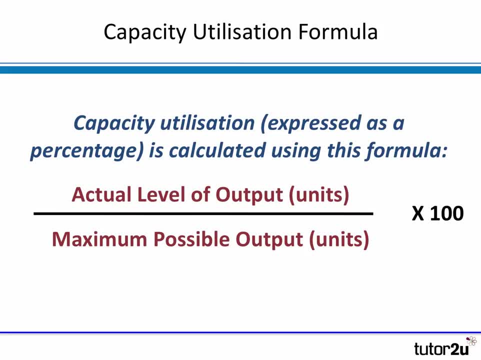 the capacity, the potential output. We calculate capacity utilisation as a percentage And the way we calculate it is to first divide the actual level of output in units, divided by that potential output, the capacity, also in units. That gives us a number. We multiply that by 100 to give us: 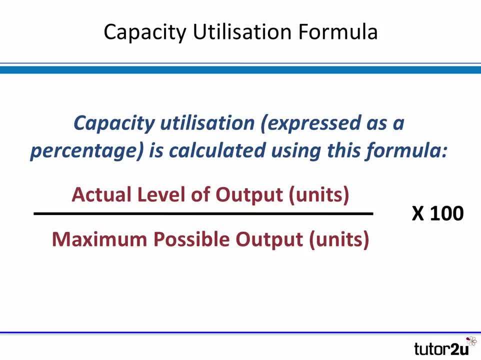 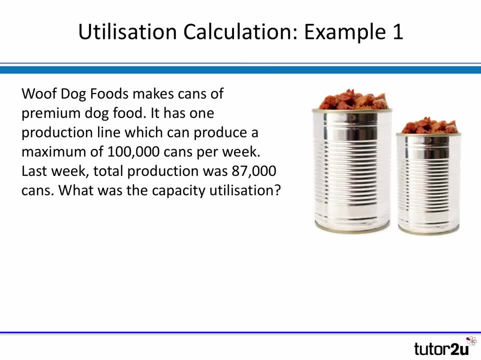 a percentage, A proportion of potential capacity that is actually used. So let's have a quick look at two or three examples of this calculation in action So you can see the different ways in which capacity utilisation can be asked. We've got a small case study here. It's a manufacturer of dog food. Woof Dog Foods has one. 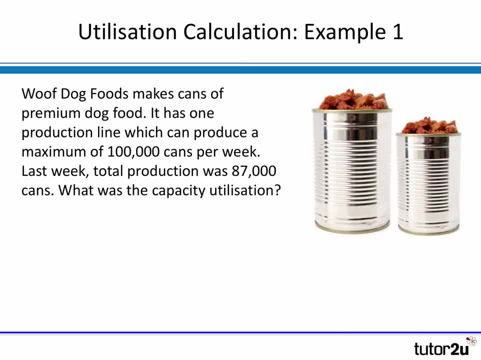 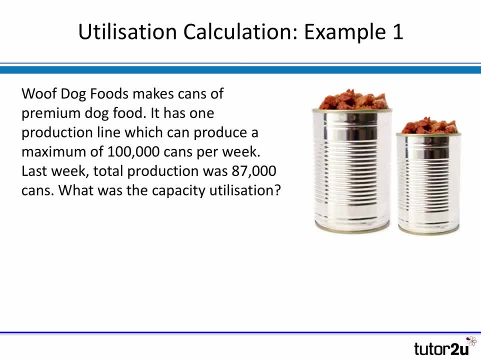 It's a measure of capacity. It's the potential output over a specified period, In this case 100,000 cans per week. That's a lot of dog food. Last week, we're told total production or actual production was 87,000 cans. 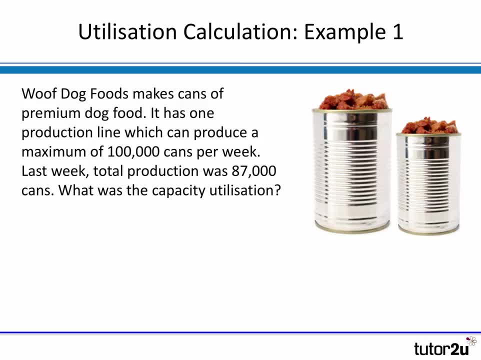 So the first question is: what was the capacity utilisation? I'll pause the video, if you wish, and have a go at calculating it. Then we'll have a look at the answer. Well, of course, we've got most of the information that we need here, haven't we? In fact? 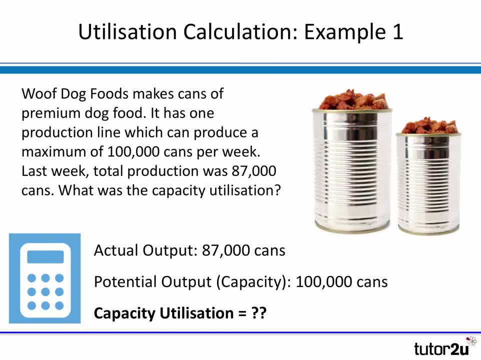 all of it. We're told the actual output of 87,000 cans. We're told the potential, ie the capacity of 100,000 cans. So we simply divide 87,000 by 100,000 and multiply it by 100. And if we do that, it comes out as 87%. 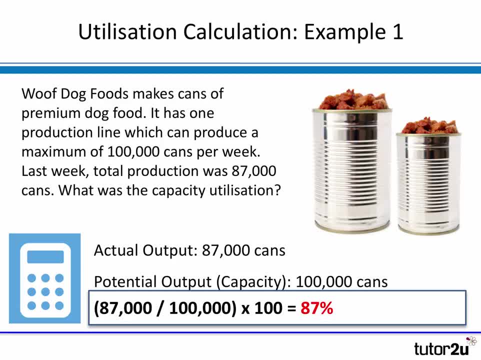 In other words, Wolf Dog Foods is operating below its potential capacity and it has spare capacity. The difference between actual utilisation and 100% of 13%, hasn't it? It could operate If it was making 100,000 cans each week. it will be operating at 100% capacity utilisation, But it's. 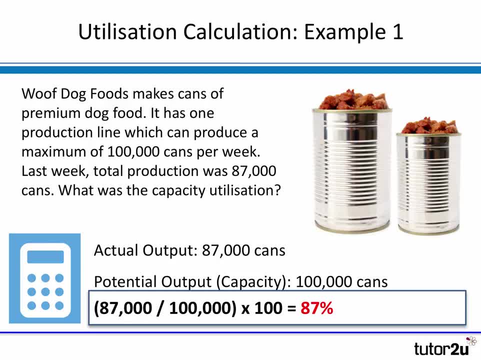 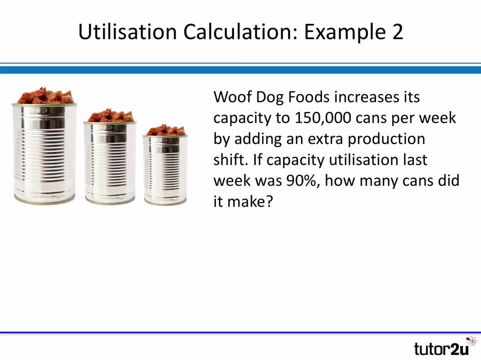 working at 13% lower than that 87% capacity utilisation. Let's just change the example slightly. We're still with Wolf Dog Foods, but now we're told good news in the dog food industry. Wolf Dog Foods has increased its capacity to 150,000 cans per week. 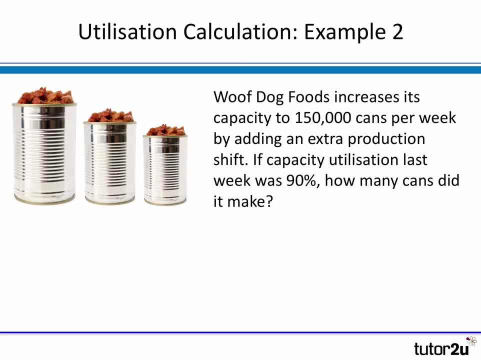 And it's done this by adding an extra production shift. If the capacity utilisation last week was 90%, how many cans did it make based on this new capacity? Have a good one, Have a good one, Have a good one. Let's take a look at the answer. We're given some of the information. we're given the potential. 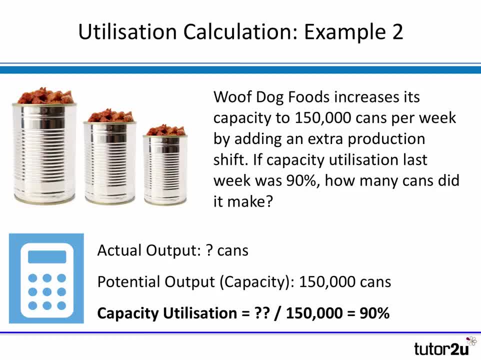 output the capacity of 150,000, and we're told that the utilisation figure was 90%. So we have to work out what the actual output was. Well, in this case, what we do is we take the potential 150%- 150,000 cans. we're told the actual output was 90% of that, So 150,000. 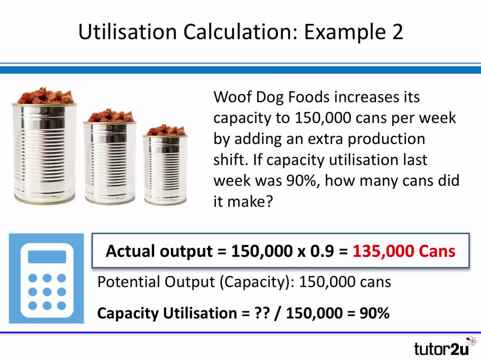 times by 0.9 or times by 90%, that comes out as 135,000 cans of dog food. So that's how many cans Woof dog food made last week at a 90% utilization rate, based on a capacity of 150,000 cans. 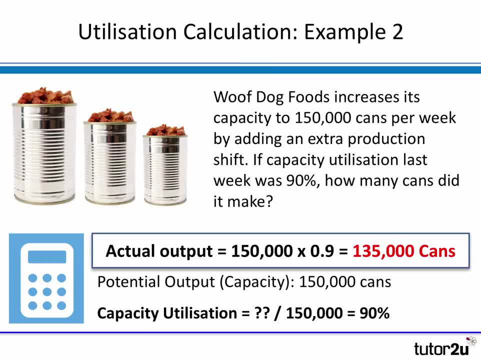 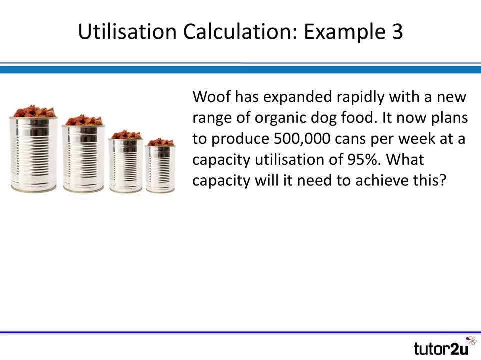 One final example just to show you the different ways in which capacity utilization can be asked. A bit more information. Woof has expanded rapidly with a new range of organic dog food. It now plans to produce 500,000 cans- half a million cans per week. 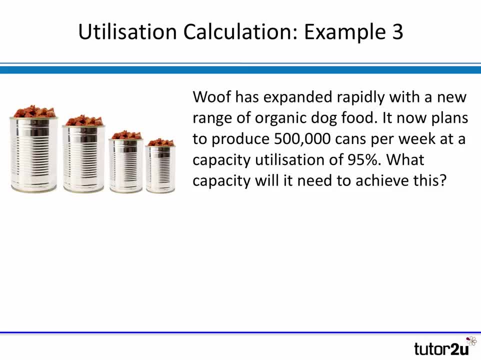 and it's planning a capacity utilization of 95%. So it wants the actual output to be 500,000 cans per week as a utilization of 95%. What capacity would it need to achieve this? Have a go at working out the answer, And if you've had a go, let's have a look at the answer. Well, we're told. 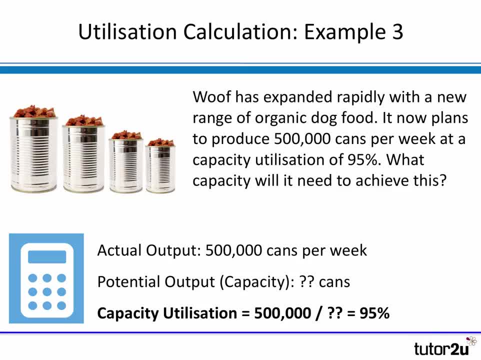 the actual output is going to be 500,000 cans per week. That's the plan. We're told that it's going to be 500,000 cans per week. That's the plan. told that the utilization needs to be 95%. In other words, we're going to need to have 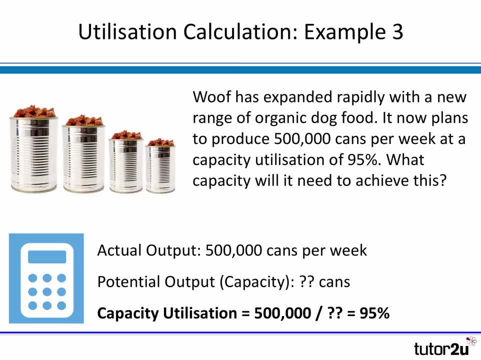 more capacity than 500,000.. How do we calculate the potential or the needed capacity? Well, it's 500,000 divided by 0.95, or divided by 95%, which comes out at 526,316 cans. So hopefully.